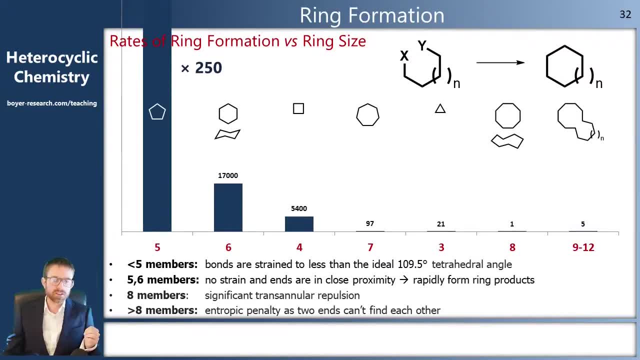 drop before the next ones. For small rings such as three, four, then there's a lot of strain to get the bonds to reach the desired angles required to make that ring. For medium size rings, so seven, eight, nine- then the reaction starts to be difficult because the 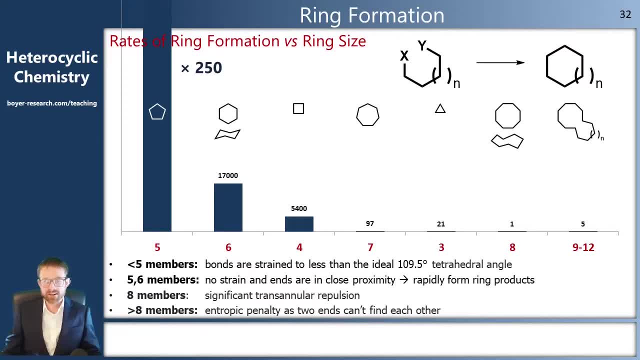 opposite sides of the ring start to hysterically clash each other. Then, finally, large rings are difficult to form because there's just no driving force for those two ends to ever meet. So it's no surprise that all of the heterocycles we'll be looking at are the five. 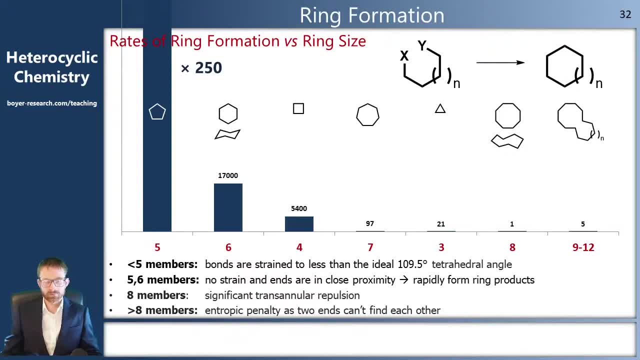 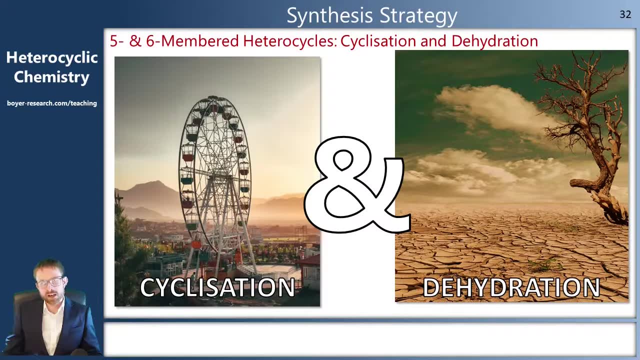 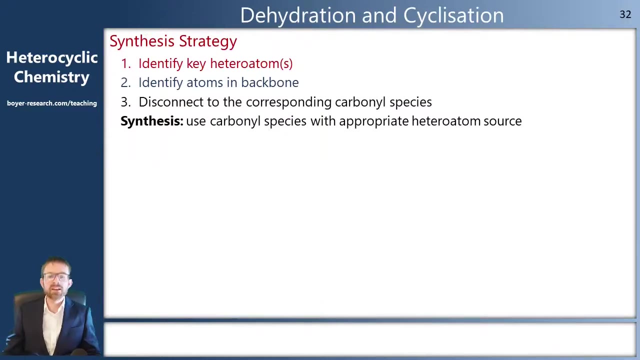 and six membered ring heterocycles. When it comes to thinking about how to make these heterocycles, well, the main strategies rely on cyclisation of acyclic molecules and dehydration, the loss of water. How do we turn this into a synthesis strategy? Well, with our three key steps. First of all, 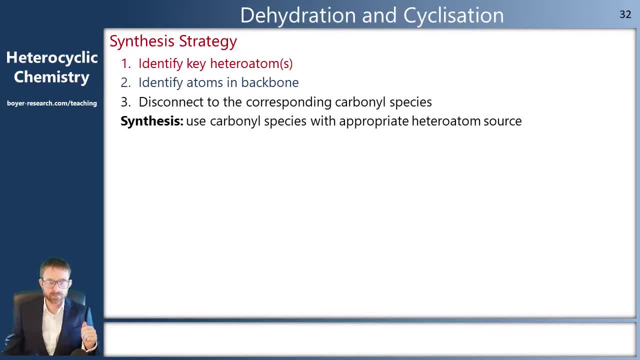 we need to identify the key heteroatom in the system. Then we need to identify the backbones around it. Finally, we need to disconnect to give a source for that heteroatom and some kind of dicarbonal species that makes up the backbone. 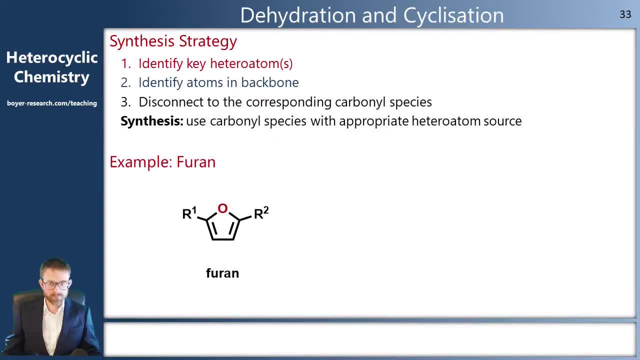 Well, what does that look like If we start off by looking at furan? there's only one heteroatom, that's the oxygen, And then that leaves us four carbons around the backbone. So if we look at the kind of four, 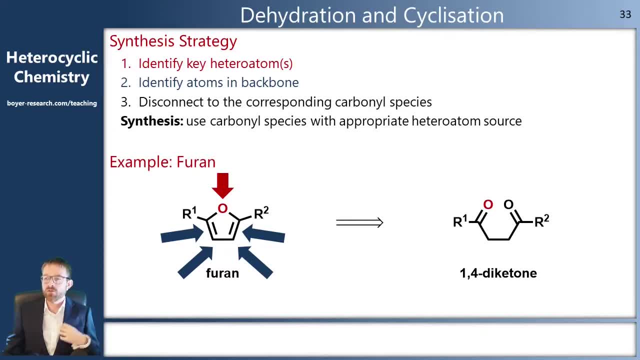 carbon dicarbonal species that we'll need. well, that's a 1,4-diketone, And because a ketone already has oxygen atom in it, that means we don't need to do anything to introduce a different heteroatom. 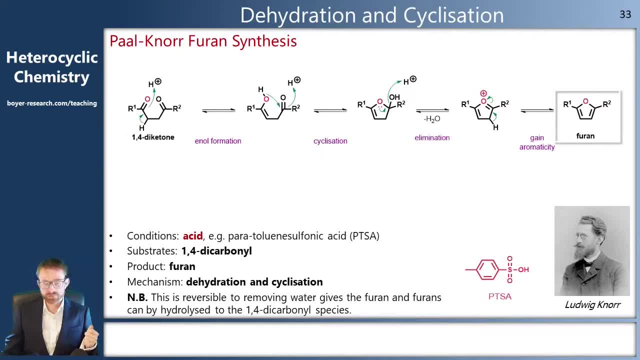 So this gives us the PAL-NOR furan synthesis, a synthesis in which, if we treat a 1,4-diketone with acid, we will promote enol-keto-tautomerization. So we can see that in the enol form the oxygen. 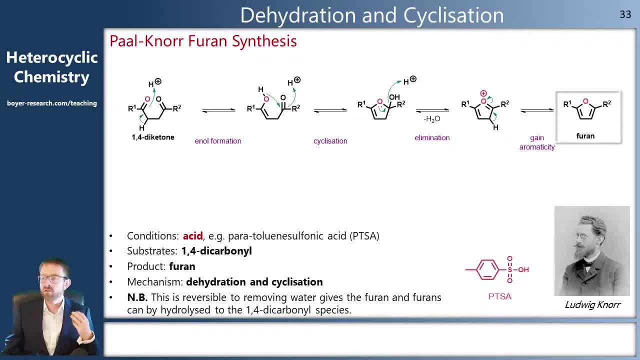 can cyclize around to form that five-membered ring, remembering that the formation of five-membered rings is very fast. And then the lone pair can assist in the elimination of water. to give the aromatic furan product Subtitles by the Amaraorg community. 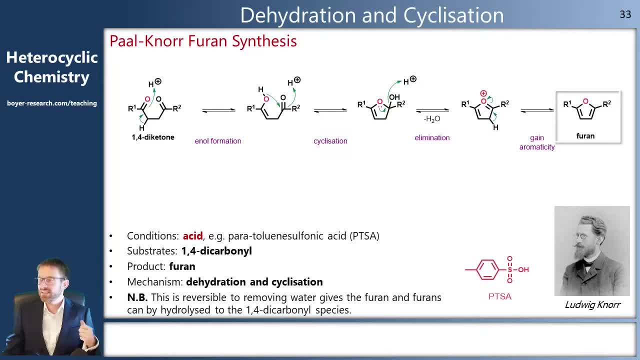 When we're looking at these syntheses under acidic conditions. there are a range of different acids which will promote this, But one of them, which we'll see quite often, is paratoluene sulfonic acid, the structure of which is shown on the screen. 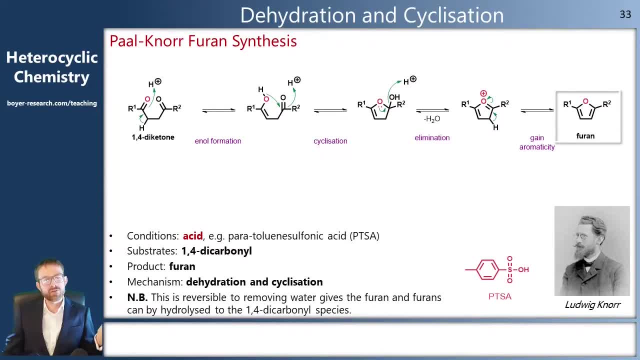 You'll note that each of these steps is reversible. So if we go from left to right, then we'll need to remove water from our reaction, And if we want to go from right to left, we'll need to add water to our reaction. 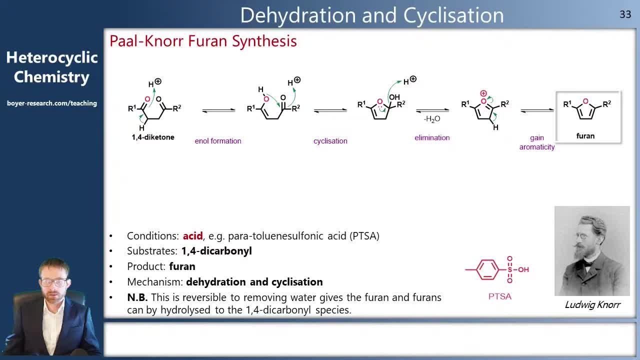 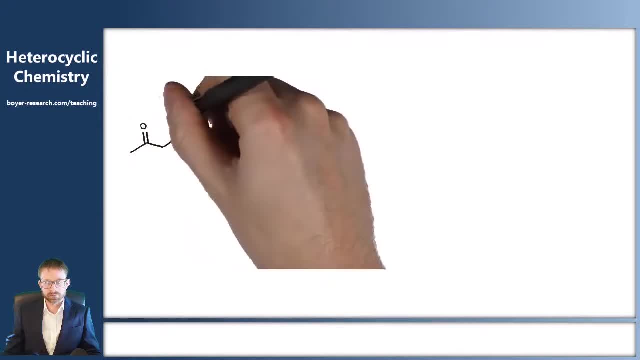 Here we go. If we look at the reaction more slowly, we'll start off with our 1,4-dicarbonyl species. That's the four carbon atoms in the backbone that will make the backbone of our furan Under acidic conditions. 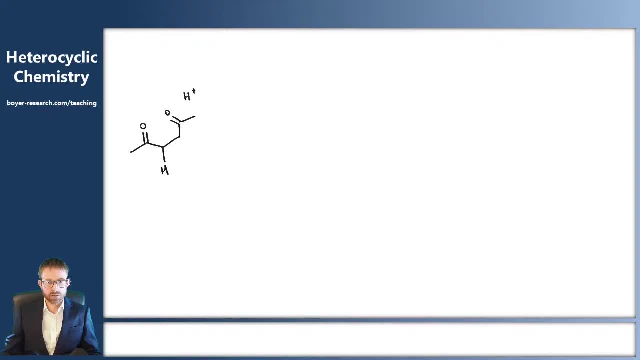 Subtitles by the Amaraorg community. We can get keto enol, total summarization, And the oxygen atom can attack the carbonyl To make the five-membered ring. Finally, we can use the oxygen lone pairs to assist with elimination of water. 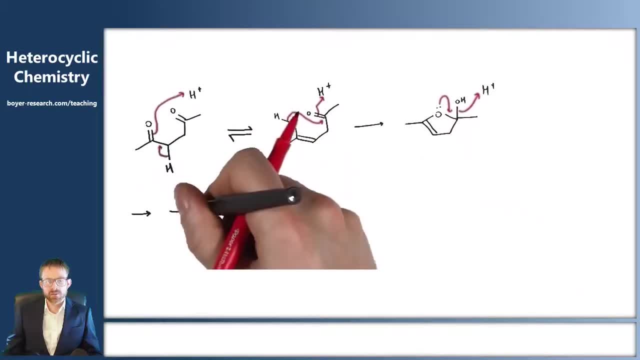 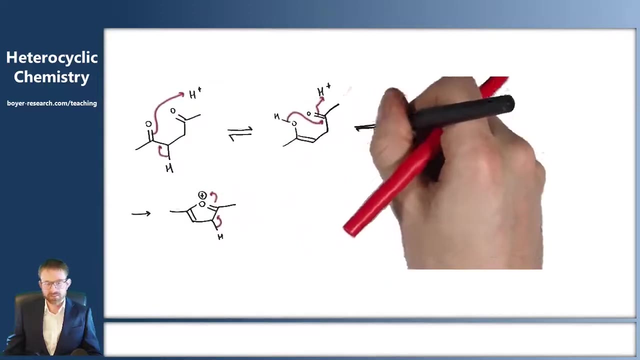 First forming an oxonium species And then, by loss of a proton, to build the aromatic system, Remembering that each of these steps is reversible, That takes us from our 1,4-dicarbonyl compound to our fuel and product. 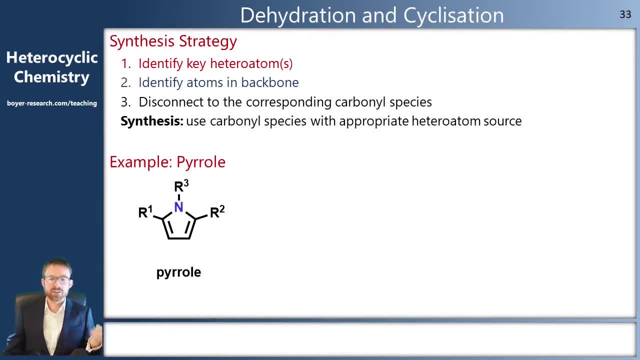 So if we want to consider a different heterocyclone Such as a pyrrole, Analyzing this shows our heteroacetamide and nitrogen. We have the same four carbon backbone And that suggests that we need some kind of amino ketone this time. 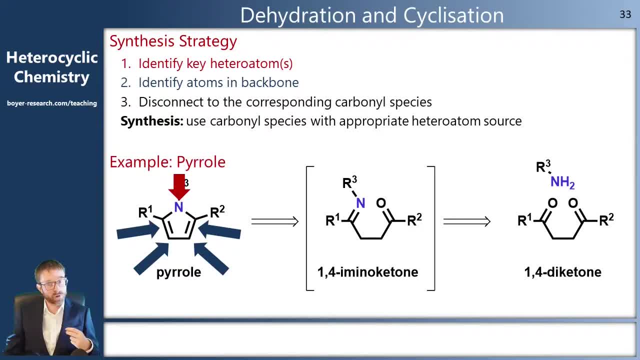 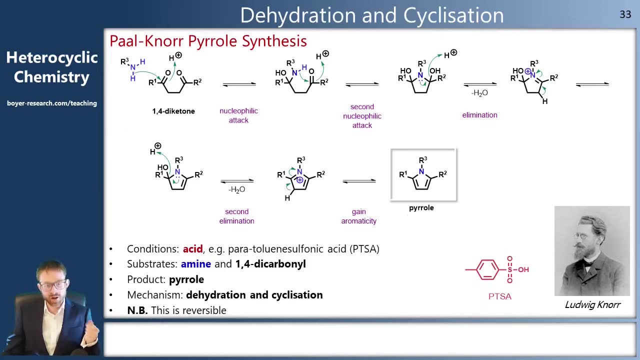 Which we will be able to get from a 1,4-diketone, same as before, This time with introduction of an amine. So, Under acidic conditions, Our nucleotides, Electrophilic nitrogen- will attack the electrophilic oxygen of one of our carbonyls. 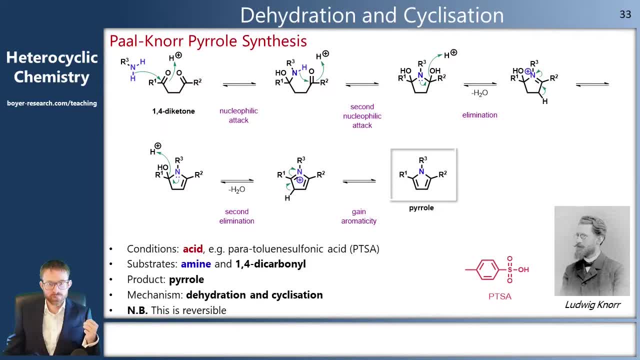 And then we'll get an attack of a second carbonyl. This will build the five-membered ring And the lone pair can come in, and it can assist the removal of water By making an iminium species, And then loss of a proton gives us the enamine. 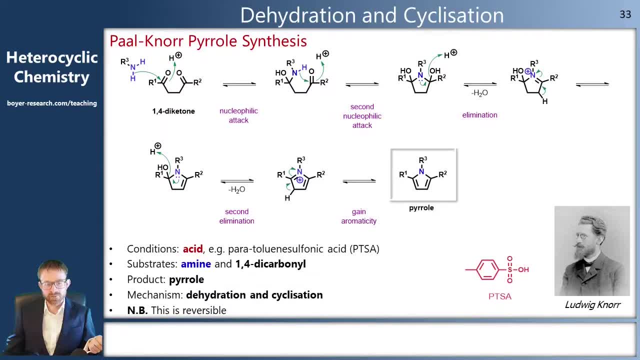 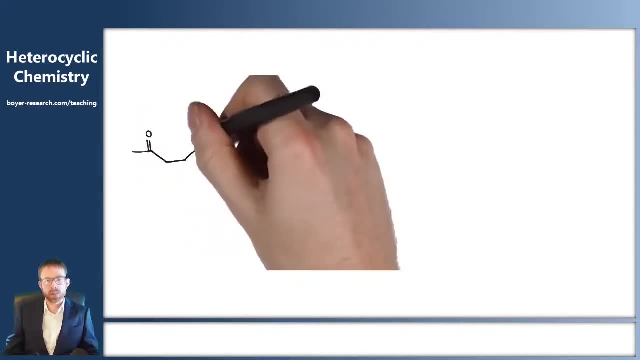 And we can do that twice To build the aromatic system. Again, this is a reversible process And again it can be catalyzed by acid. If we look at it in a little bit more detail, We have our key 1,4-dicarbonyl species. 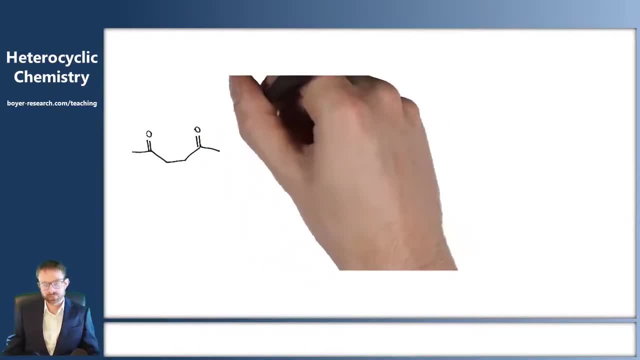 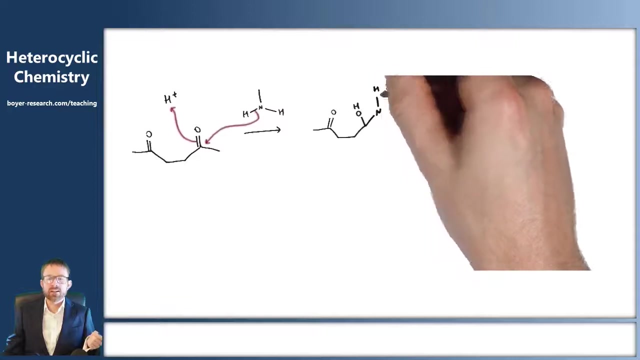 And our amine. that provides us the nitrogen that we need for our pyrrole. The acid will activate And our acid will bounce back. That will help activate the carbonyl so that our amine will attack, but then our amine is still reactive. 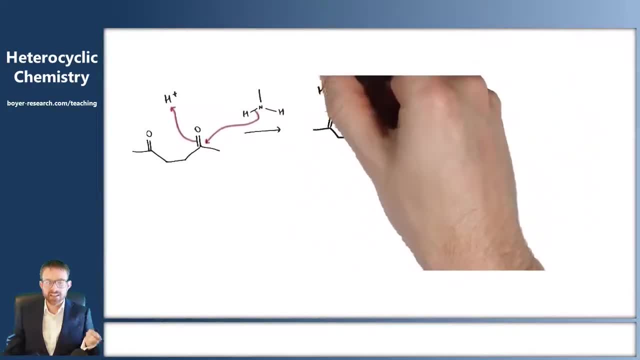 and we still have acid and we still have a second carbonyl. so we can get the second attack to make our five-membered ring, which is a very fast ring form to size, ring size to form, and that gives us our five-membered ring and this double hemi-aminole style intermediate. 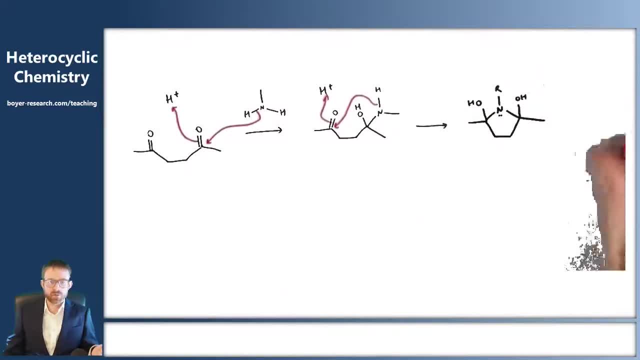 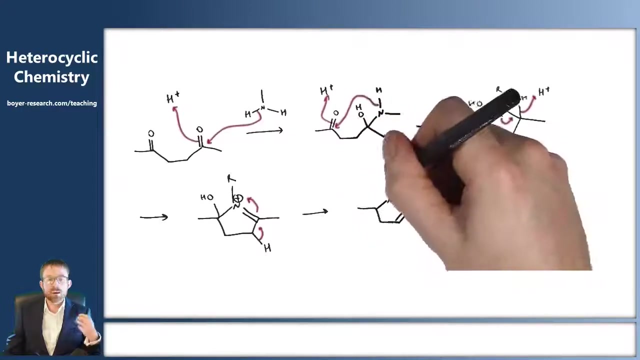 We can use the nitrogen lone pair to assist with the elimination of water. so it pushes in, we lose the OH, assisted by the acid, and then we lose a proton to give us our enamine. We can draw the exact same thing again and that results in the loss of our second molecule of water. 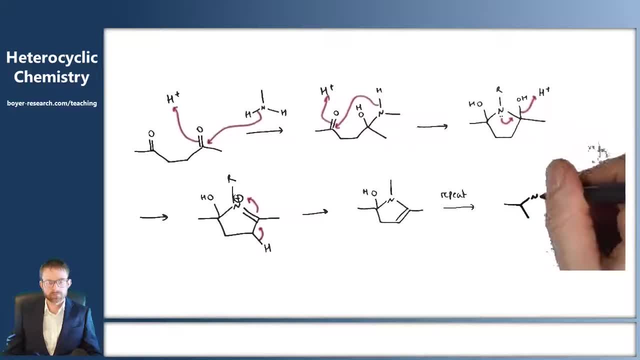 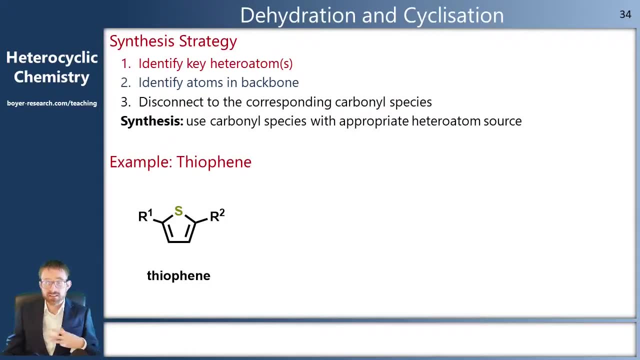 and the formation of our aromatic pyrrole. So let's continue. Instead of a nitrogen or an oxygen, if we want the sulfur, so a thiophene. again, we need to find where we're going to get the sulfur atom from, and again we're going to have four carbons in the backbone. so we need a diketone, a 1,4-diketone. 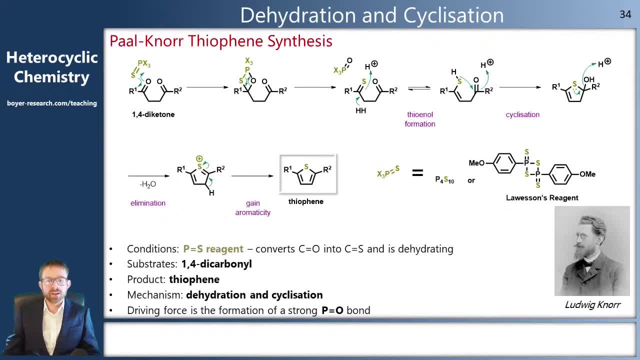 and some kind of source of sulfur. Well, for this we're going to use a phosphorus-sulfur reagent. So this is a reagent which has a phosphorus-sulfur double bond. Several times now we've seen how phosphorus reagents are very oxophilic. So what this? 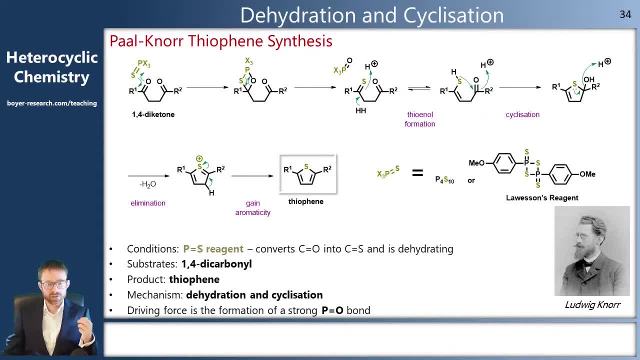 reagent will do is it will swap its phosphorus-sulfur double bond for the carbon-oxygen double bond in our substrate, And so you can see here, it swaps the ketone for a thio-ketone, Again following the exact same mechanism, at this stage, as for the furan synthesis. 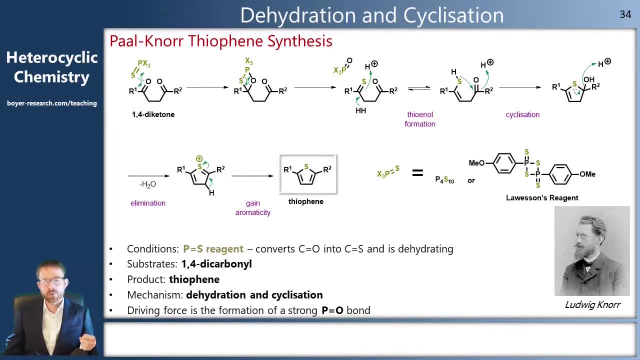 we can form the sulfur equivalent of the enol-keto-topical polymerization: intramolecular attack and then elimination of water. This gives us the aromatic thiophene, and one of the reagents that we're going to use is a pyrrole. 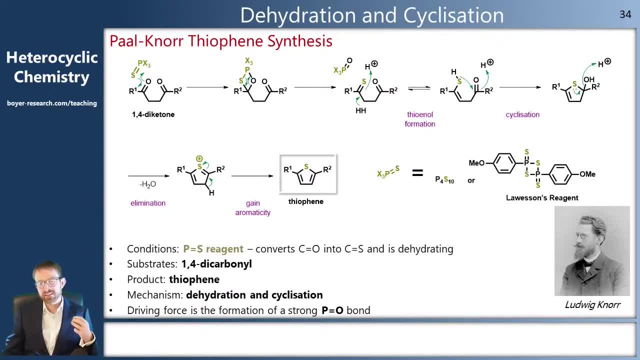 So we're going to use a pyrrole. So we're going to use a pyrrole. One of the reagents that we can use for this is Lawson's reagent, which is shown on the screen, or P4S10.. 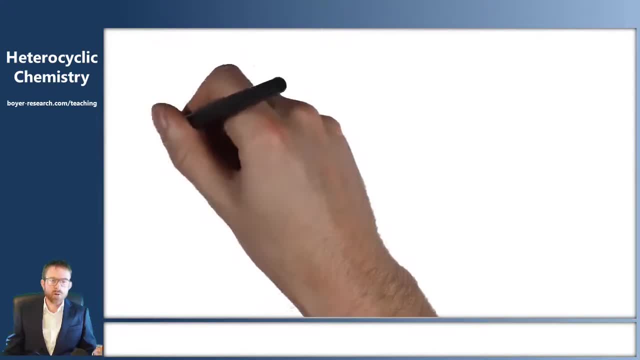 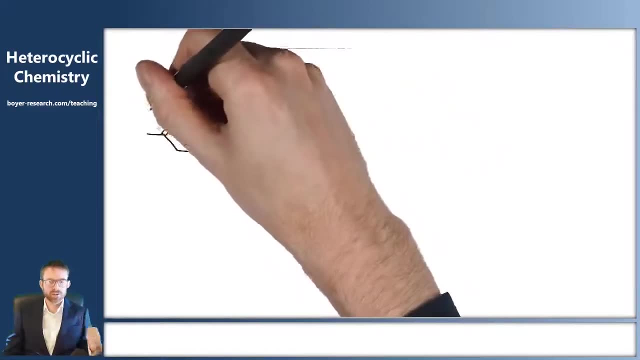 So the key element of this is our 1,4-dicarbonyl, which we're getting very used to seeing now, But we need to swap out the oxygen for sulfur, And so we're going to use a phosphorus-sulfur reagent. 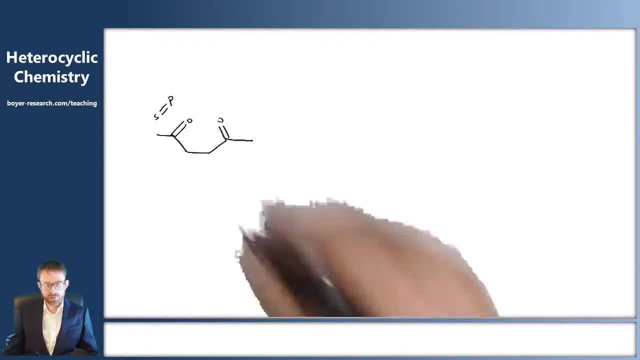 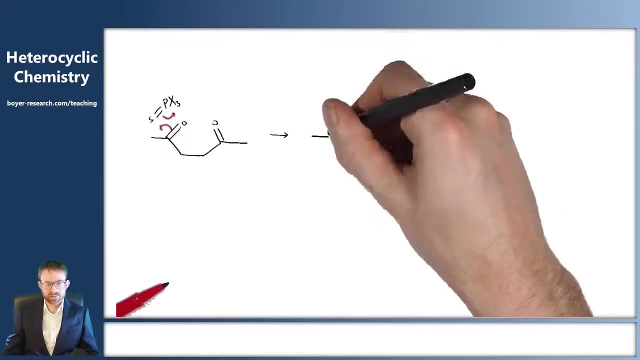 The driving force will be the formation of a phosphorus-oxygen double bond, And so we can draw arrows which swap that sulfur for the oxygen. We form an intermediate four-membered species that makes the first phosphorus-oxygen bond. Then, by pushing the same arrows again, we complete the process. 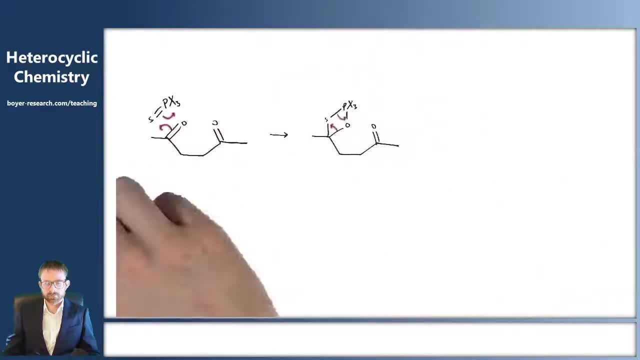 And form a thioketone. Our thioketone will come and attack our carbonyl Again. five-membered ring is very quick to form, so this is a good transformation And this leaves us an OH. The sulfur-blown pair can come in. push that OH out. 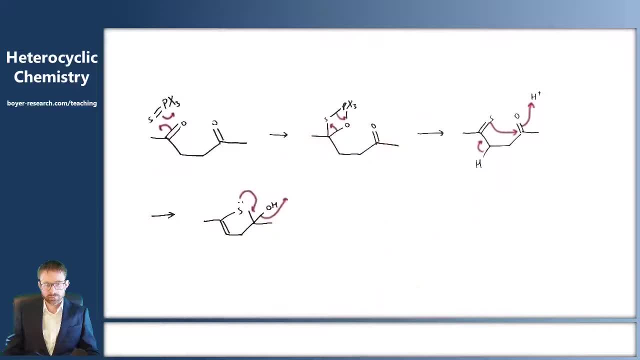 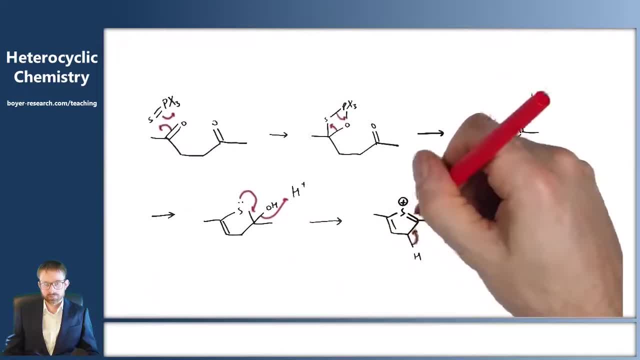 Thyoketone, Thyoketone, Thyoketone, Thyoketone, Thyoketone, Thyoketone. This strategy doesn't just work with five-membered heterocycles. We can look at six-membered heterocycles. 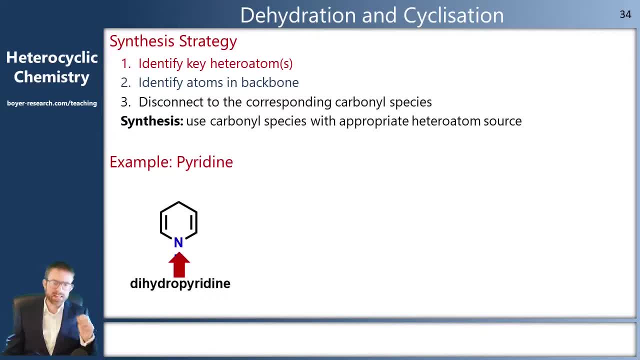 So if we, for example, look at a dihydropyridine again, our key heteroatom is the 9-membered. That meet for our monoclonal nit�ardon is the 3-numbered, The 0 is a 2: 1 Yar service. week夜 service. 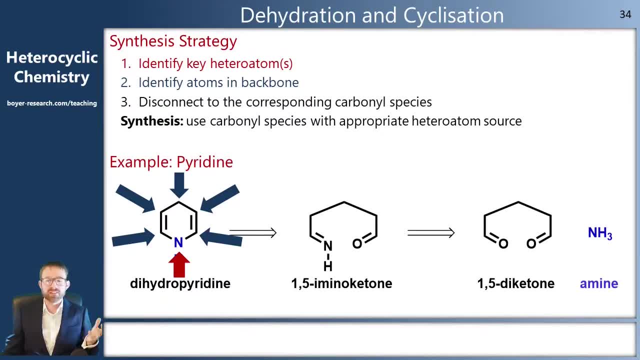 And that stands for. one dose may not have singleota 1.. It's not that it prep boom, But it's really about landing a focus on the Bill names. So now we need to look for what five-membered heterocycles in the backbone. 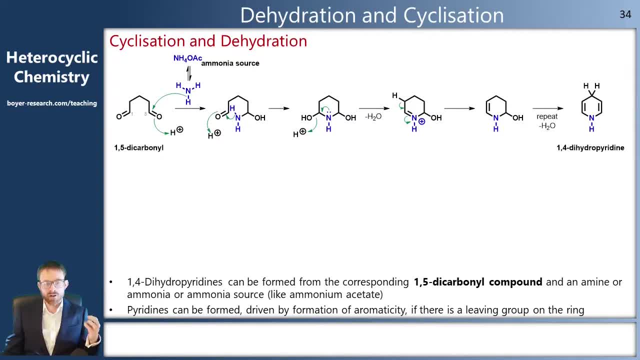 And that now gives us five carbons in the backbone. So now we need to look for a 1, 5appinginoketone, which will come 1, by carbonyl and an amine source in very much the same mechanism as the synthesis our nuclear nitrogen. 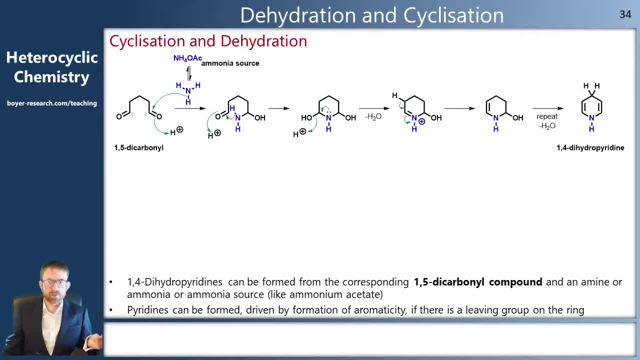 linen will attack each one of our carbonyl And then we'll get loss of water to form the double enamine species. However, this time, because it's not a 5-iridine, we will not end up with the aromatic system and we'll end up with a 1,4-dihydropyridine. 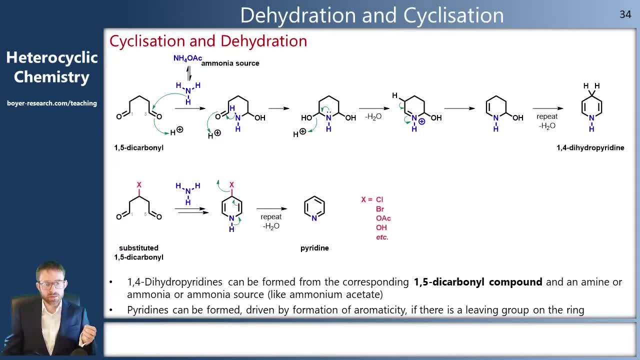 But if instead of a 1,5-dicarbonyl species we have a 1,5-dicarbonyl species with some kind of leaving group on the backbone, so here represented by X, where X could be a. 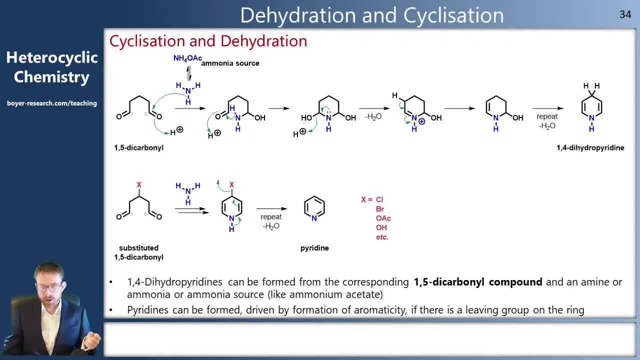 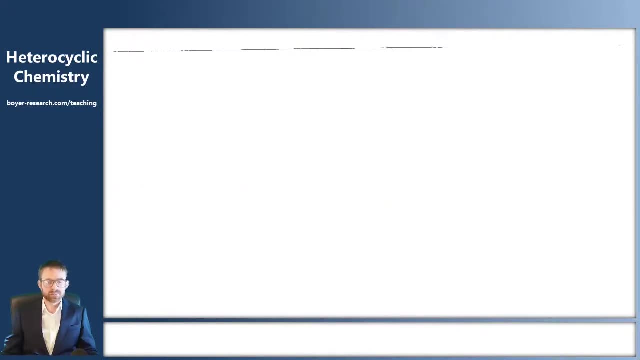 chloride, a bromide, an acetate, etc. well then, at the end of this sequence, we could get the formation of the aromatic system by loss of HX. Looking at this in more detail this time, because it's a 6-membered ring, we need 5. 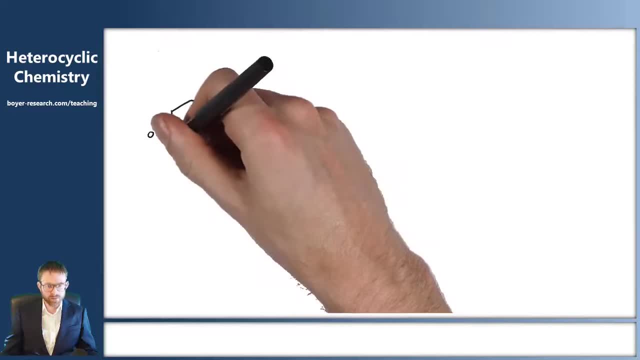 carbons, and that will come from our 1,5-dicarbonyl, And we need a source of ammonia. Ammonia is a gas, so we'll have to use something like ammonium acetate if we want to use it in the laboratory. 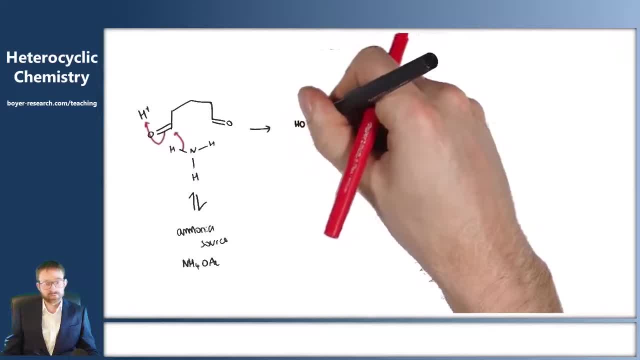 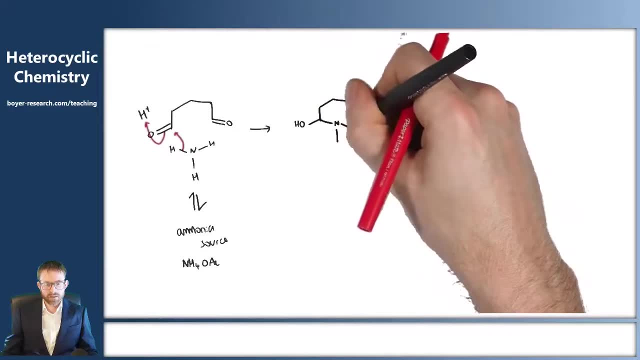 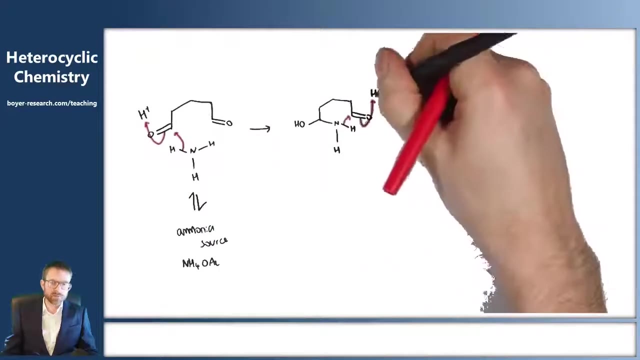 And our nucleophilic nitrogen attacks our electrophilic carbonyl. And it not only does this once, it does this twice, this time, making it a 6-membered ring, which is slightly slower than a 5-membered ring, but it's still extremely favourable. 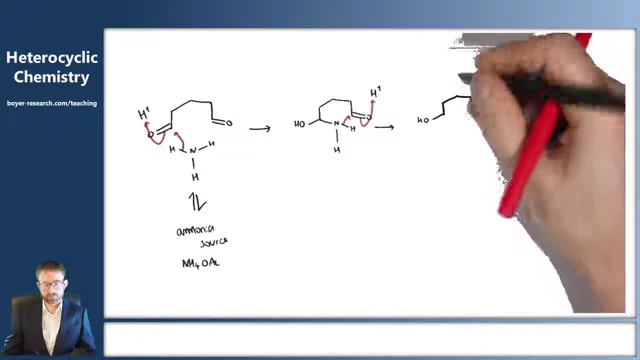 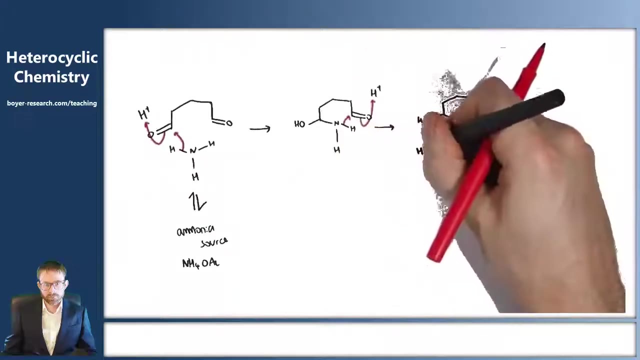 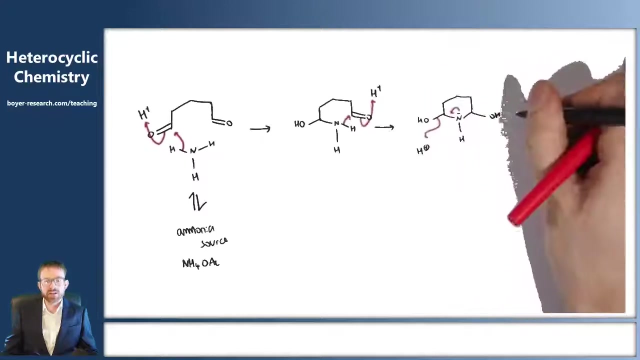 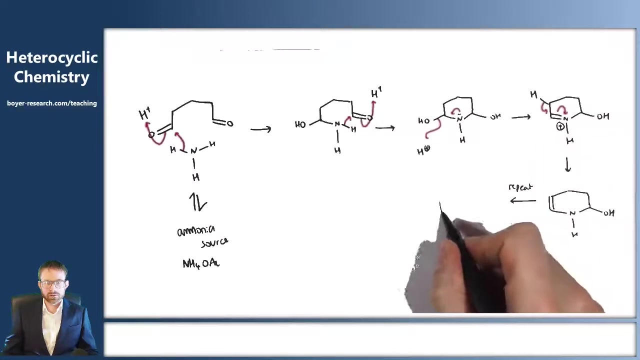 We can repeat that process on the other side and that gives us R1, 4-dihydropyridine. 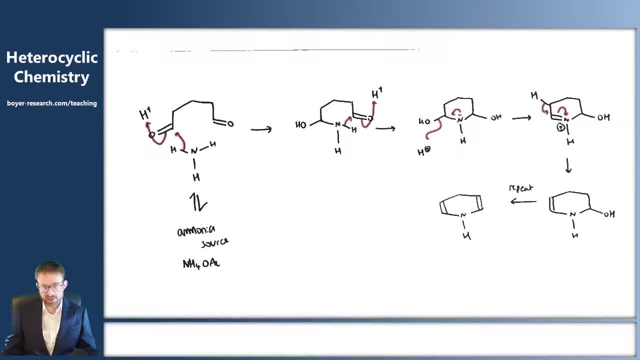 So the pyridine, but with an extra hydrogen at the 1,, ie, nitrogen and the 4 positions. But if our 1,, 4, 5-dicarbonyl starting material has some kind of leaving group in there, 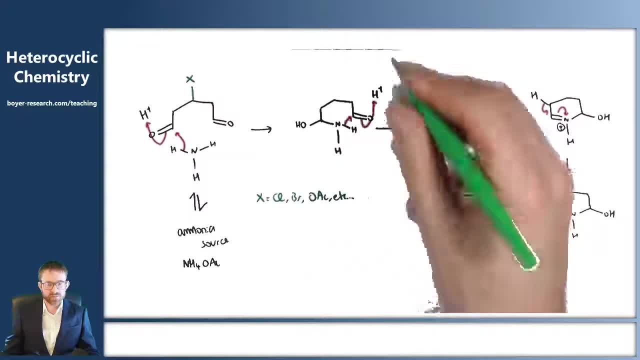 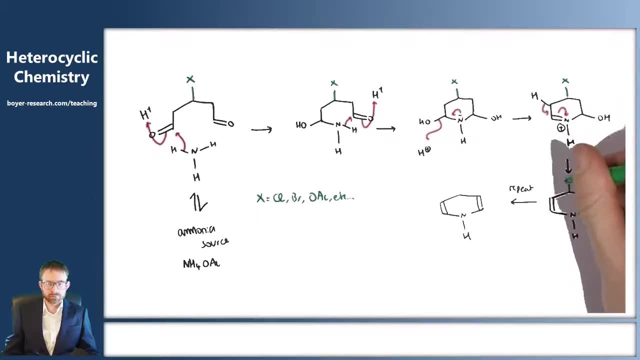 so X, where X is a halogen acetate, OH, etc. well, we can draw the exact same mechanism, following the X, all the way through the process And then, in the final step, we'll get loss of HX from our system. 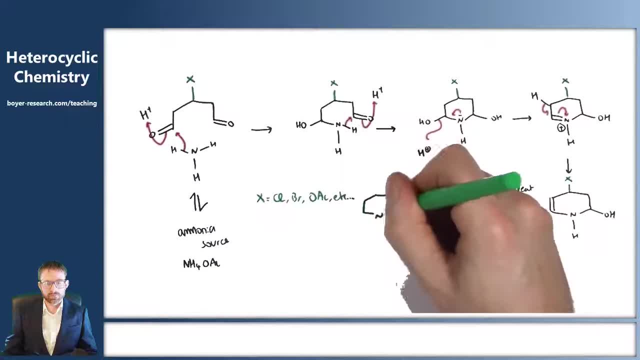 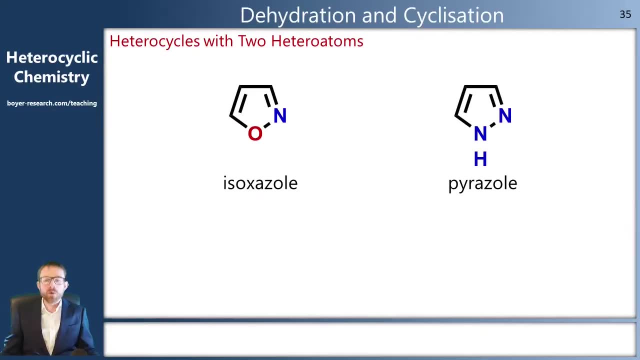 And B, We can build the aromatic pyridine. Alternatively, if there is no X, we could use an oxidant that we've seen in an earlier video. What do we do if there is more than one heteratom? Well, the system still applies. 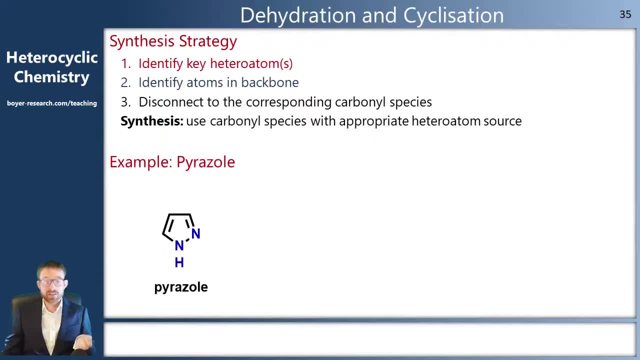 So if we look at a pyrazole, we now need to identify the key heteratom, but this time there's two of them, So we have the two nitrogens, which leaves us a 3-carbon backbone. So this time we're going to need a 1, 3-dicarbonyl. 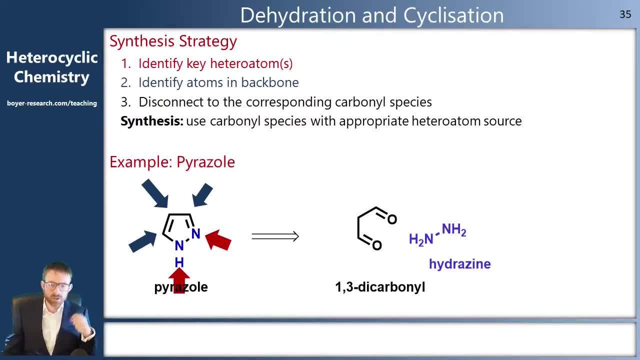 and a source of O2.. So we're going to need two of those two nitrogens And two nitrogens with a single bond between them. two NH2s with a single bond between them is called hydrazine. 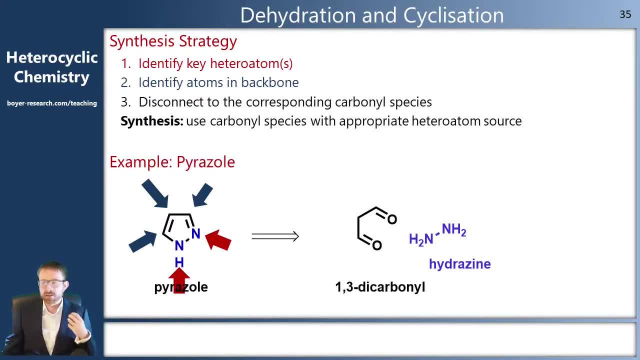 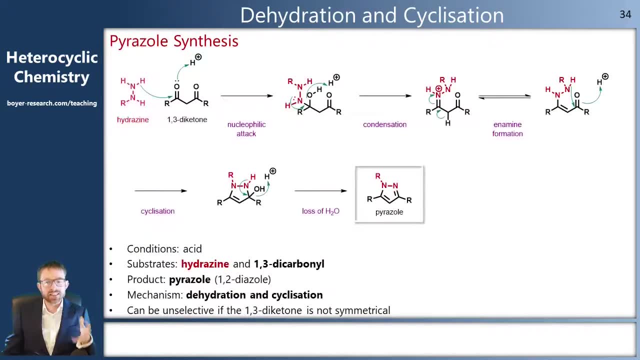 Hydrazine is very nucleophilic because the lone pairs of each of those two nitrogens repels each other, therefore making an already nucleophilic nitrogen atom even more nucleophilic. In a similar mechanism, we activate our 1, 3-dicarbonyl species with acid. 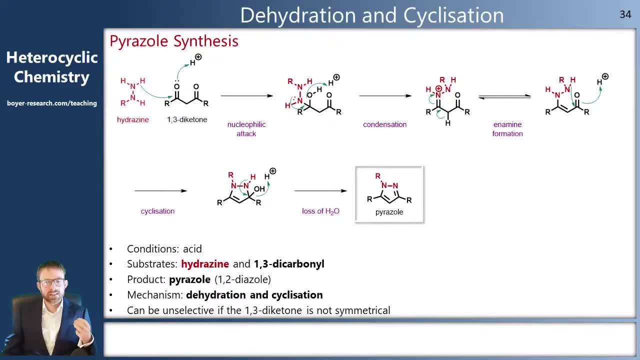 and our nucleophilic nitrogen attacks. This time our lone pair comes in and it promotes the loss of water and we get a neutralisation of the resulting iminium to form an enamine. Intramolecular cyclisation of the second nucleophilic nitrogen onto our electrophilic carbonyl. 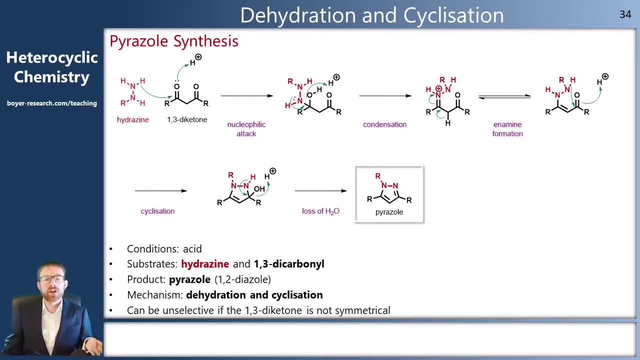 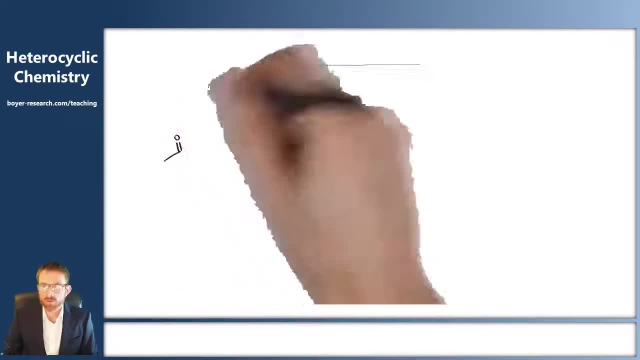 promoted by acid, then completes our 5-membered ring, followed by loss of water to give us the aromatic product. So we start off with our backbone, which is our 1, 3-dicarbonyl species, and our heterosome source, which is a hydrazine. 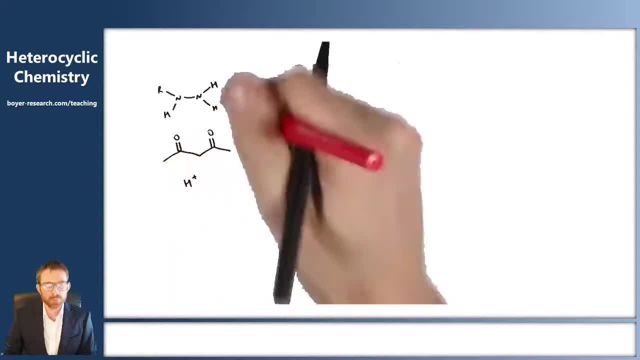 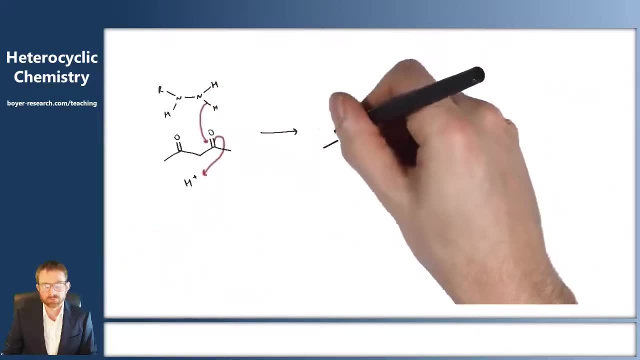 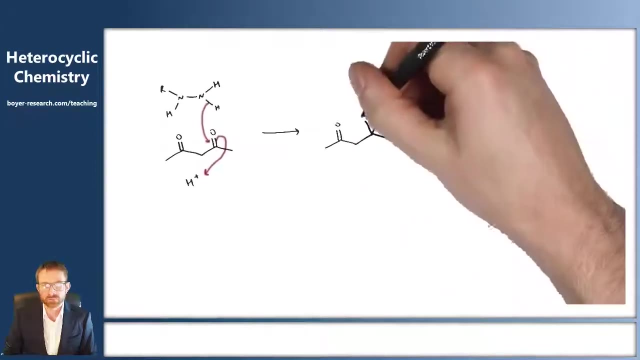 The hydrazine is very nucleophilic, and so it will attack our electrophilic carbonyl promoted by acid. This forms the first carbon-nitrogen bond that we'll need for our heterocycle if we have to do 보통. 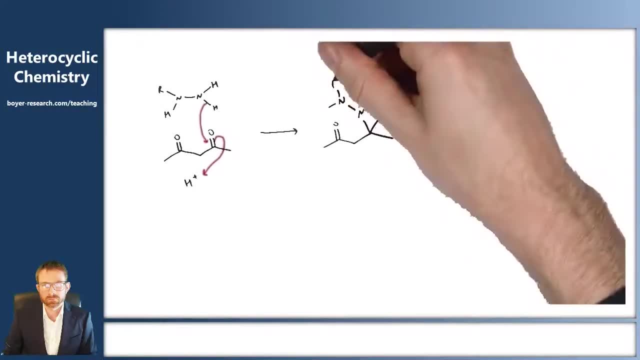 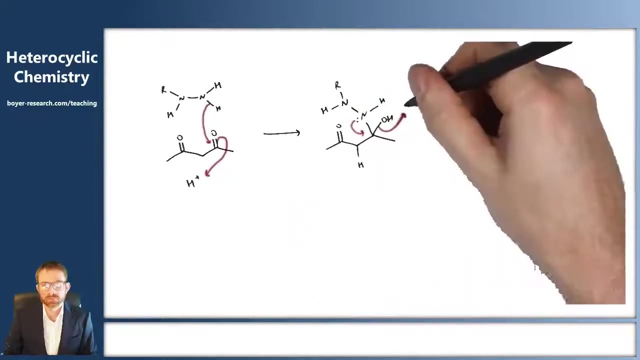 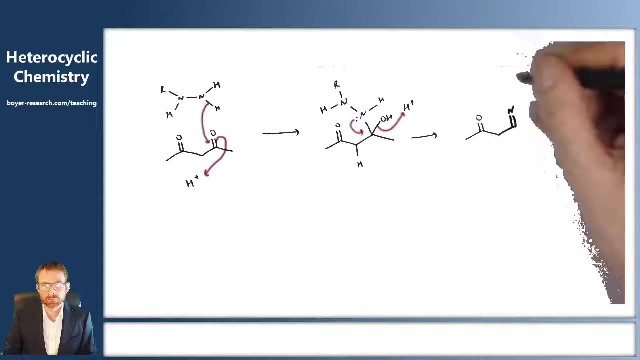 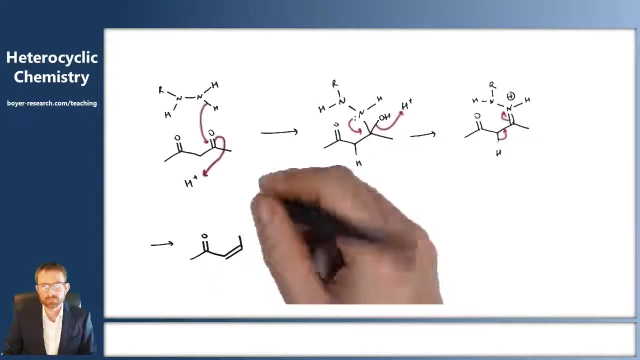 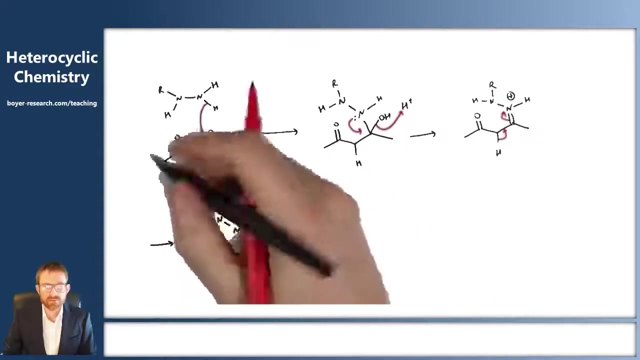 an readership of carbon-nitrogen 1, 3-dicarbonyl RL of 0,. And then loss of hydrogen will give us the enamine. The second nitrogen can rapidly cyclise to make our five-membered ring, attacking the 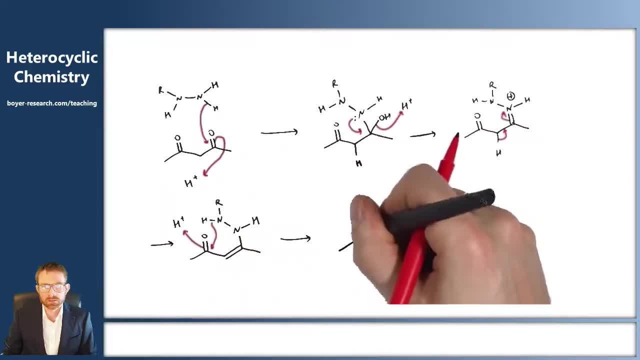 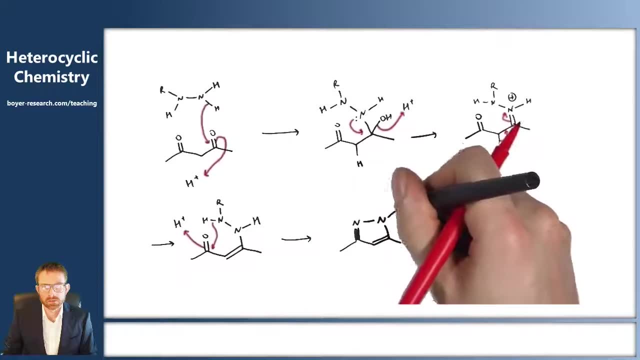 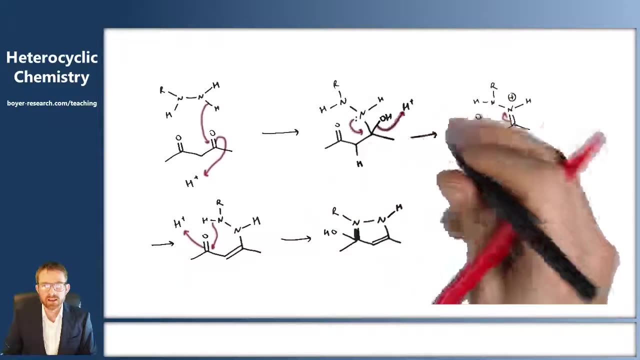 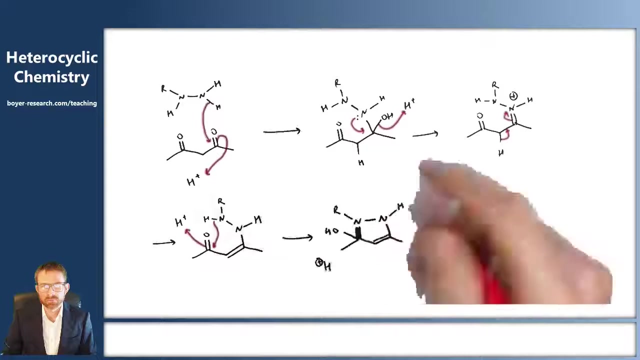 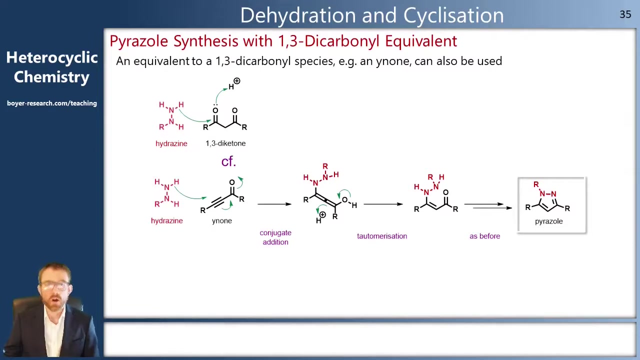 electrophilic carbonyl. And then, finally, a second elimination of water, promoted by a nitrogen-burned pair. This will give us the aromatic heterocyclone. In addition to 1,3-dicarbonales. we can actually consider other molecules which have similar. 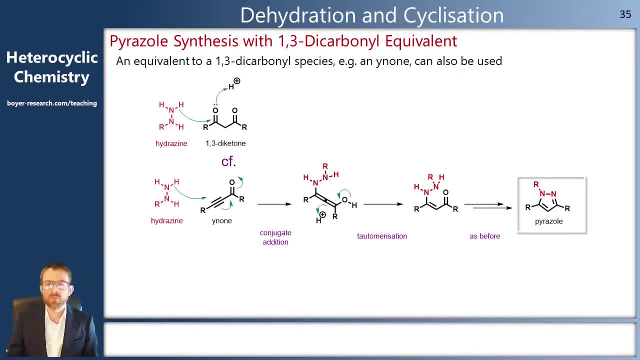 properties. So here, for example, instead of a 1,3-dicarbonate carbonyl, we can see that the hydrosome could do a conjugate addition to an inone. So the 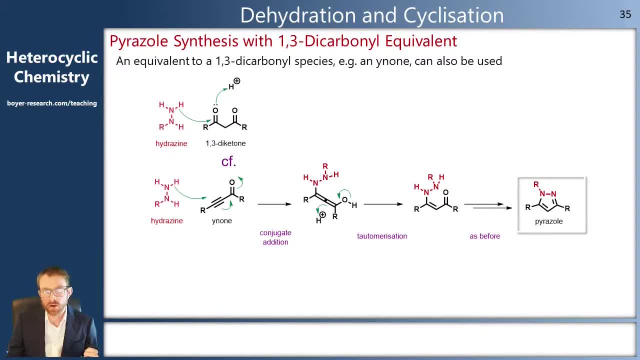 inone is behaving the same as our 1,3-dicarbonyl, Because after that first conjugate addition, we end up with the exact same intermediate as we've seen for this process. So it's worth pointing out it's not just 1,3-dicarbonyls that can take place in this, but also 1,3-dicarbonyl. 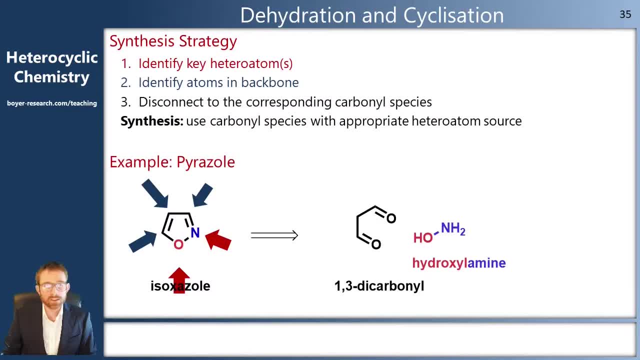 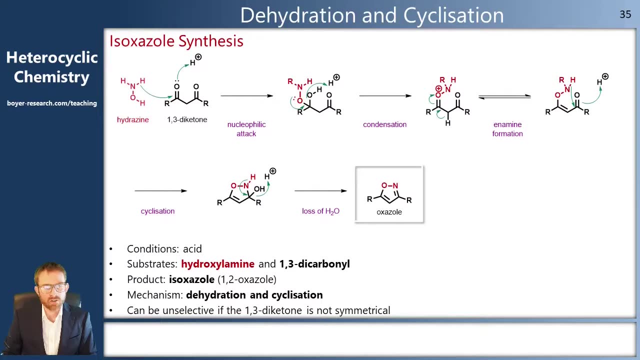 equivalents such as inones. We can also do analysis for isoxazole, This time instead of hydrazine we can just do the hydroxylamine. The mechanism is identical, but now we have the attack of an oxygen and a nitrogen separately, But we can flow it through from our hydroxylamine. 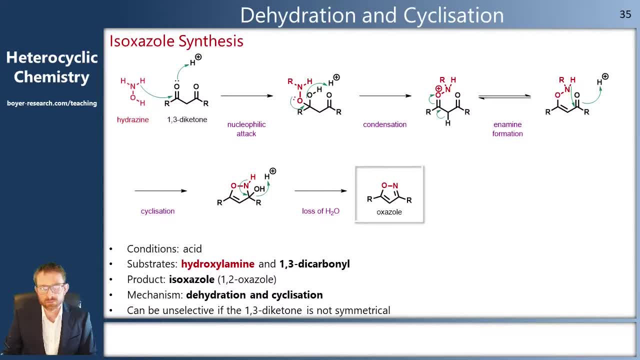 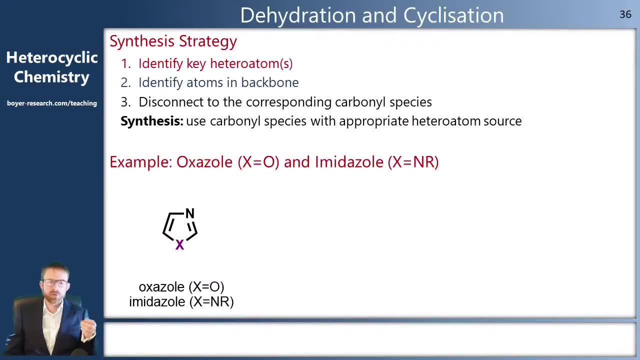 to our oxazole product. What happens when our heteroatoms are not next to each other, So, for example, using oxazoles or imidazoles? Well, again, we can apply the same strategy. However, this time we're going to look. 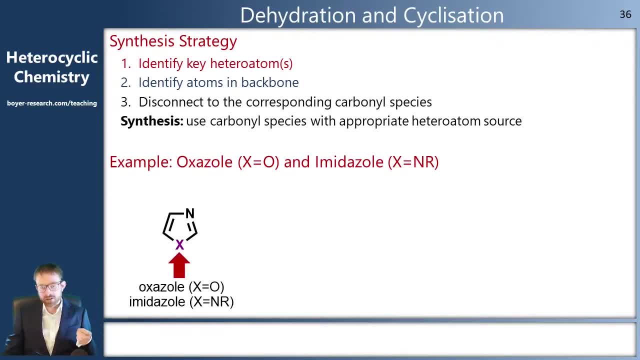 at our key heteroatom, which is the X. So in oxazole, that's an oxygen, and in imidazole, that's an NR group, And the backbone is going to contain a different heteroatom. So the N is built into our backbone this time. 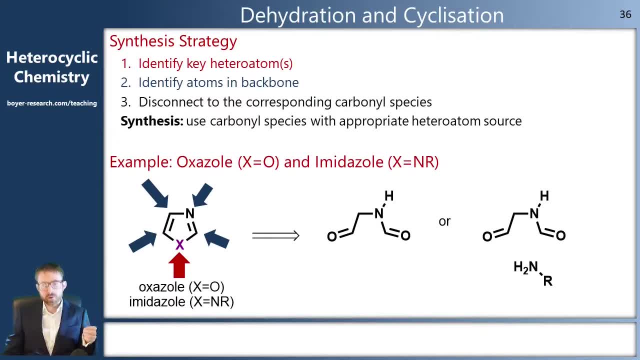 Which means that instead of a 1,4-dicarbonyl or a carbon species, that means there's a nitrogen in there. So if we want to make the oxazole, we can just take the 1,4-dicarbonyl directly If we want to. 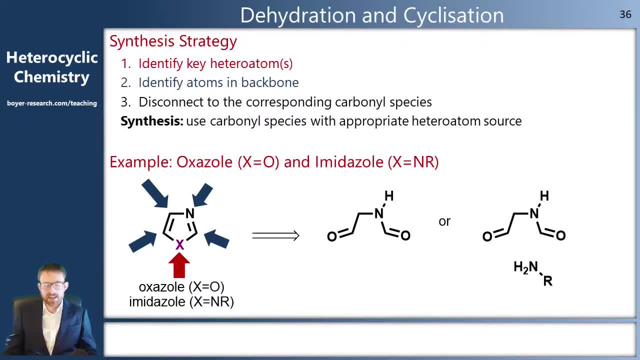 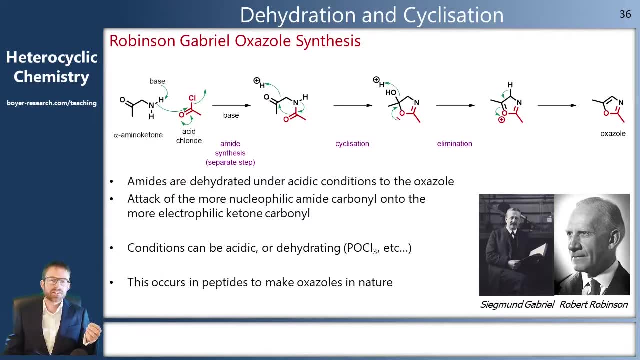 to make the imidazole, we're going to have to take the 1,4-dicarbonyl and mix it with an amine. So this is a Robinson-Gabriel synthesis and you can see that starting from a readily available 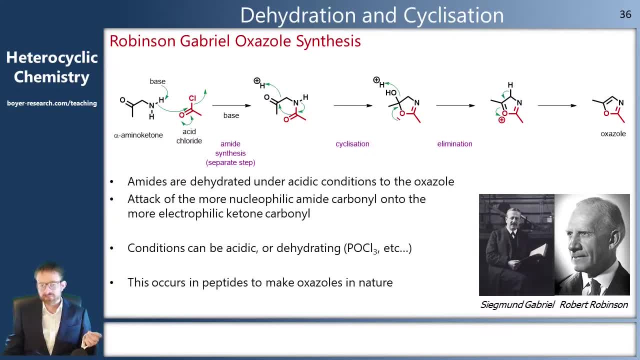 alpha-amino ketone. we can react that with an acid-chloride to give us this backbone. so it's very easy to make the kind of backbone that we need then if we treat that with acid. our electron-rich amides is electron rich because the nitrogen lone pair is in conjugation with the carbonyl can. 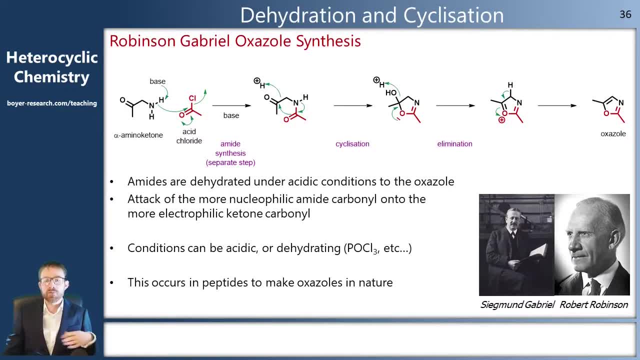 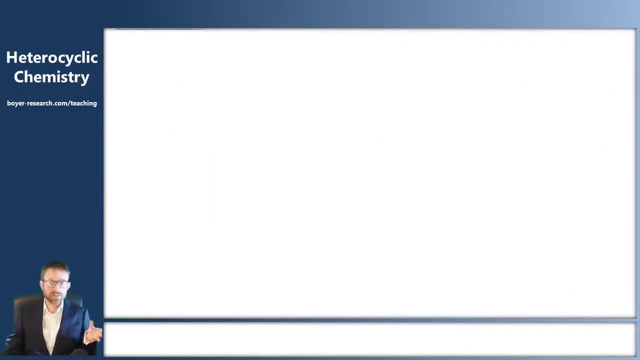 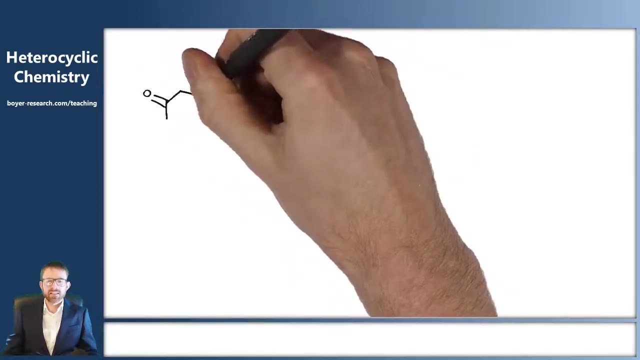 attack our electrophilic carbonyl promoted by acid. this makes that five-membered ring. then an oxygen lone pair can come in, promote the loss of water to give us our aromatic product. so our starting materials are easy to synthesize. we have the formation of an amide in the labs. we will typically do. 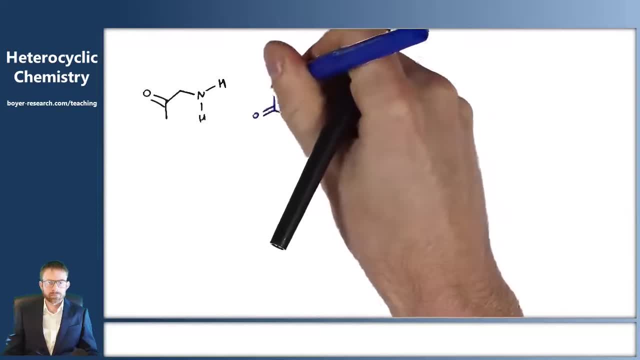 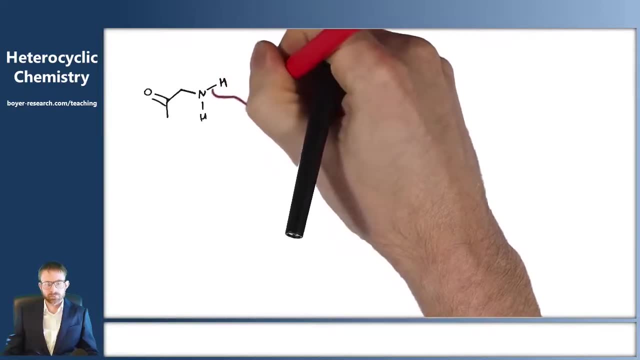 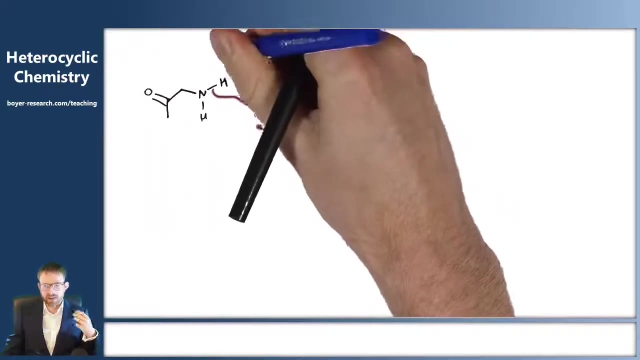 this with an acid chloride and an amine. but in nature there's a lot of amide bond formations and proteins etc. so we get nucleophilic attack promoted by a base of our nucleophilic nitrogen onto our acid chloride. we push the electrons up onto the oxygen, then back down to lose. 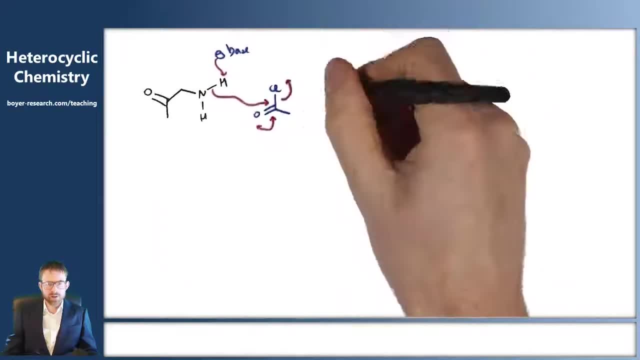 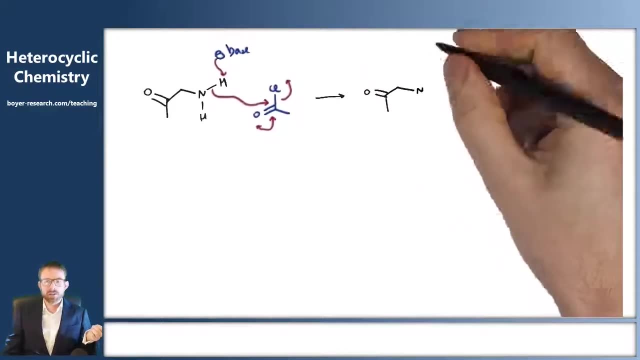 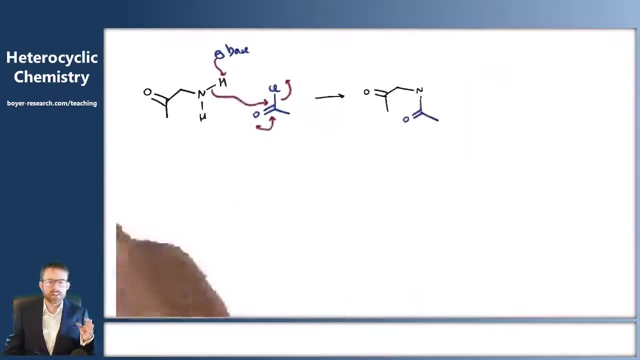 chloride and give us our new nitrogen carbon bond. this is our key one for dicarbonyl species, for our oxazole synthesis. we can draw the electron rich, carbonyl, more electron rich now because of nitrogen lone pair which is in conjugation, so it's the amide which is 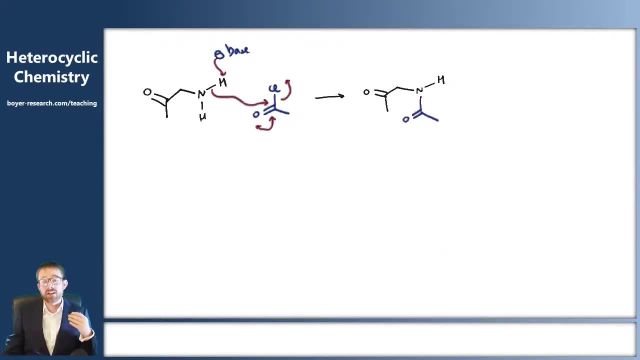 electron rich- the cyclase is round and reacts there- more electrophilic ketone carbon. then the next variable will be an oxygen pair- this will promote the loss of water- and is北, a hydrogen pair which is in conjugation. so this will be our oxygen. 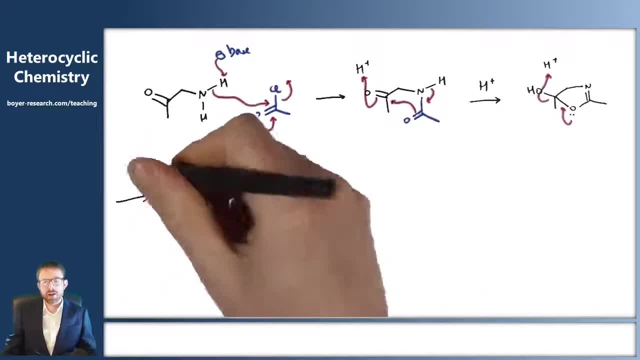 pair which is in conjugation. so this is our oxygen pair, where we can promote the loss of water by kicking out our OH promoted by acid and neutralizing this. the loss of water by kicking out our OH promoted by acid and neutralizing this with every cell of our oxygen pair. a oxygen pair will give us a high plaque in the 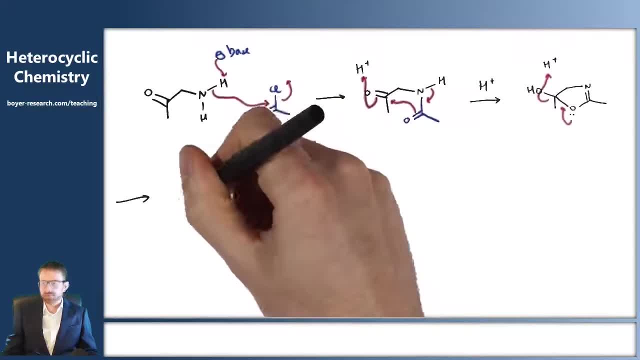 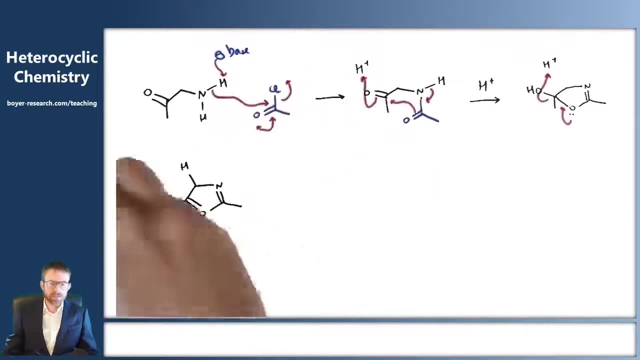 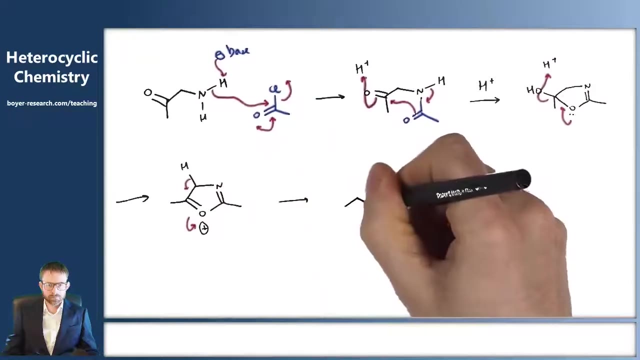 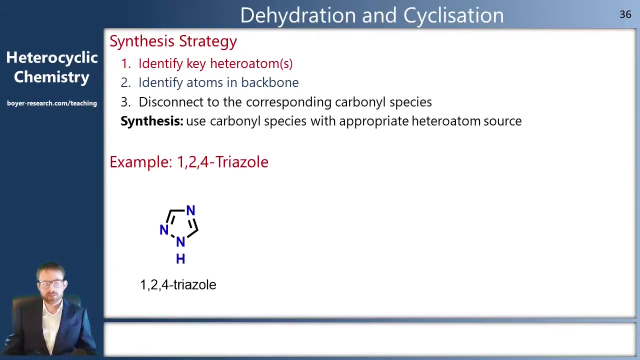 most identical group, then this is the difference between acid and nitrogen. we can, of the resulting oxonium species, builds our aromatic system and completes the synthesis of our oxazole. We can continue this and look at the synthesis of heterocycles with 3 heteroatoms in it. 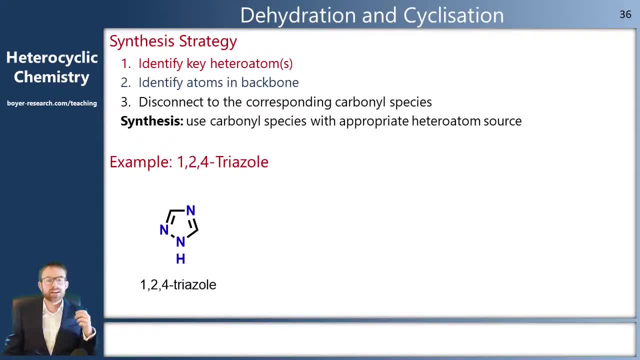 Looking at a 1,2,4 triazole, we can choose 2 heteroatoms and that leaves us 3 atoms in the backbone Again, this time there will be 2 carbons and 1 nitrogen, so we'll have a dicarbonyl species. 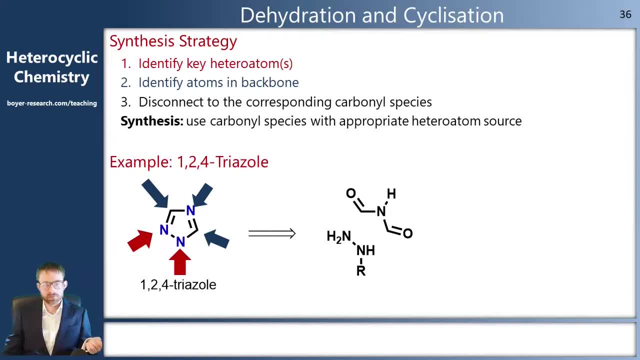 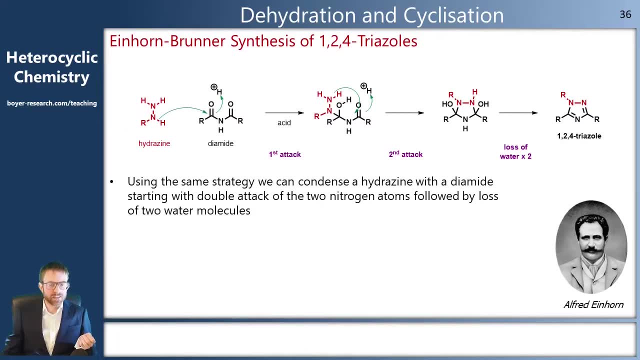 with a nitrogen in the middle and a hydrazone type species. This gives us the Einhorn Brunner synthesis, in which our nucleophilic hydrazine will attack our electrophilic diamide. then the other nitrogen from the hydrazine will attack the 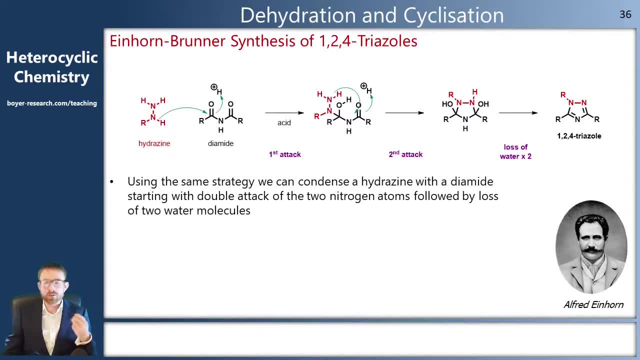 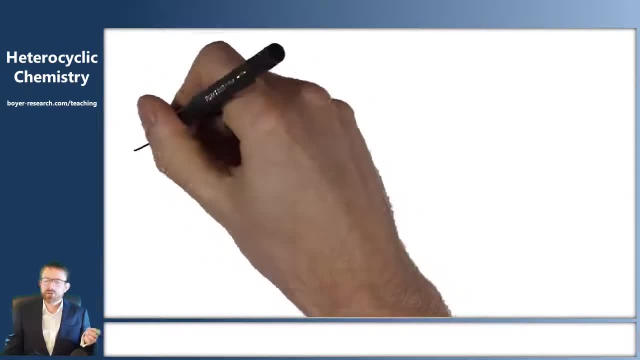 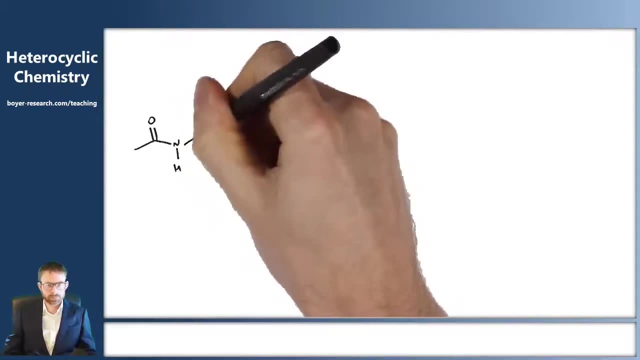 other carbonyl and finally, by loss of water, will build the totally aromatic system. So it's a very similar mechanism to what we've seen before, but with more heteroatoms in the backbone. We have our diamide, We have our hydrazine. 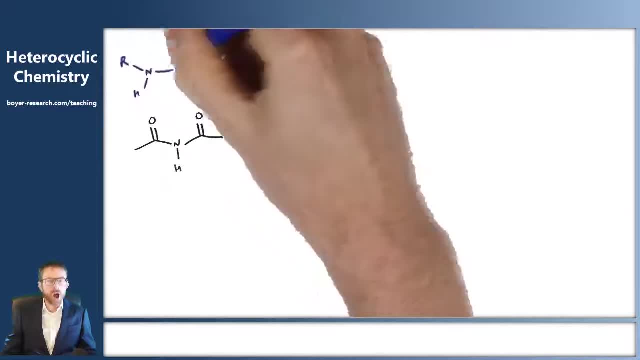 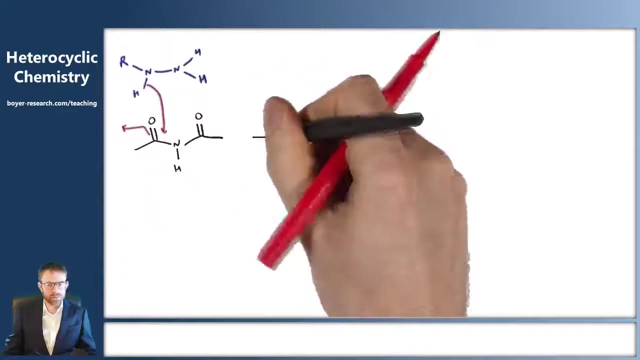 We have our hydrazine. Our nucleophilic nitrogen is going to attack one of the carbonyls of our amide. That builds the first of the two nitrogen-carbon bonds that we need. We have our amide, We have our dicarbonyl. 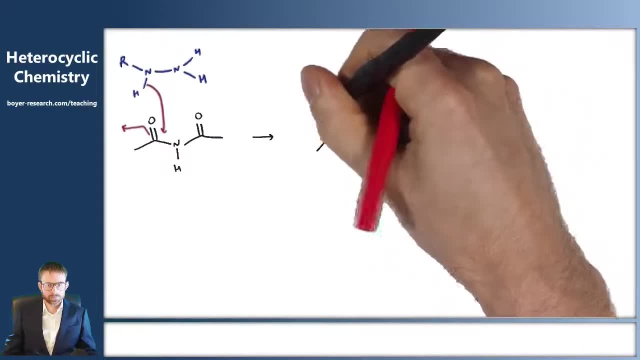 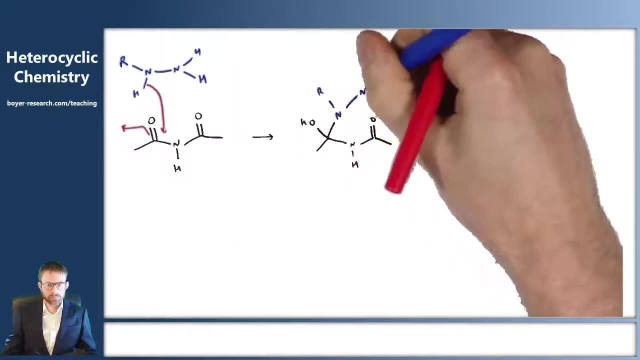 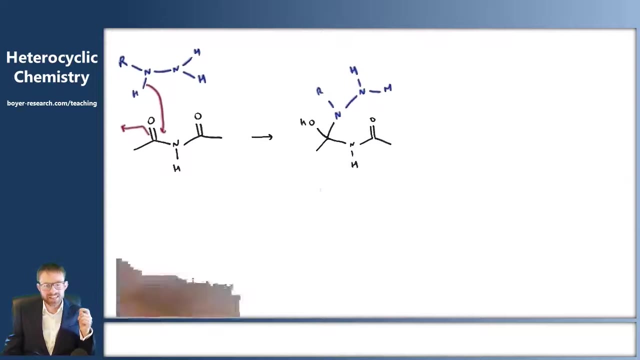 We have our amide, We have our dicarbonyl, Then the second nucleophilic nitrogen can attack the second electrophilic carbonyl and that completes the five-membered ring part of our synthesis. And that's the end of our synthesis. 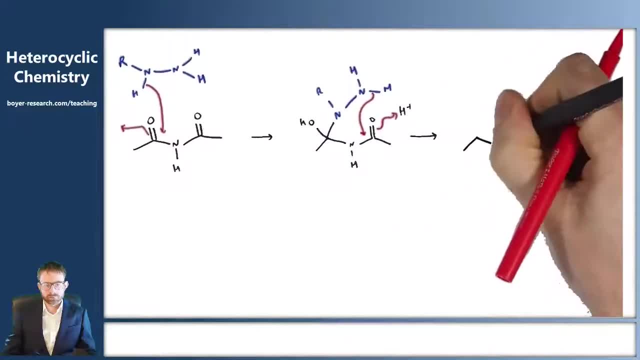 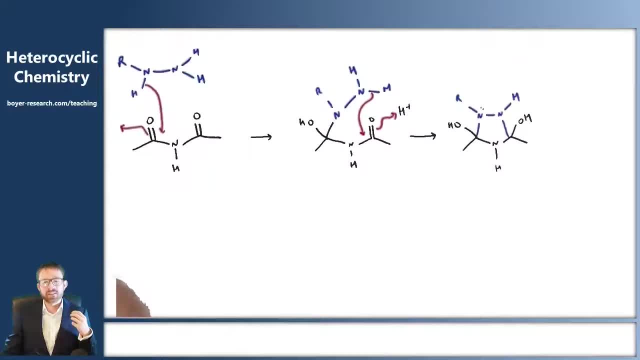 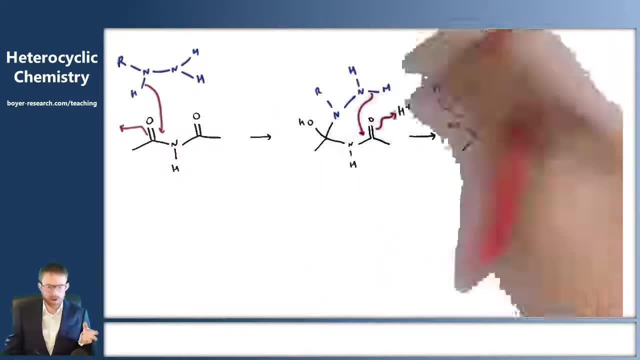 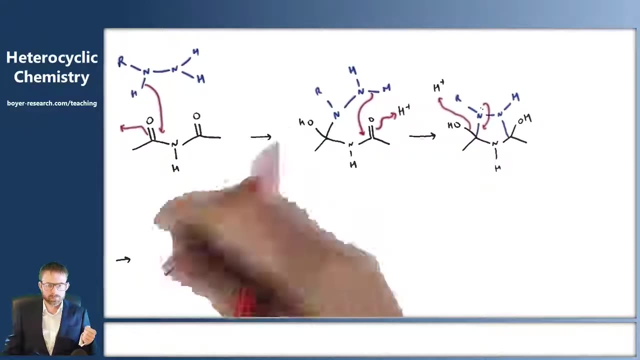 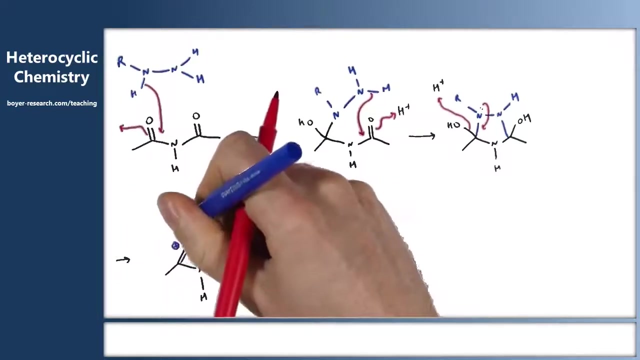 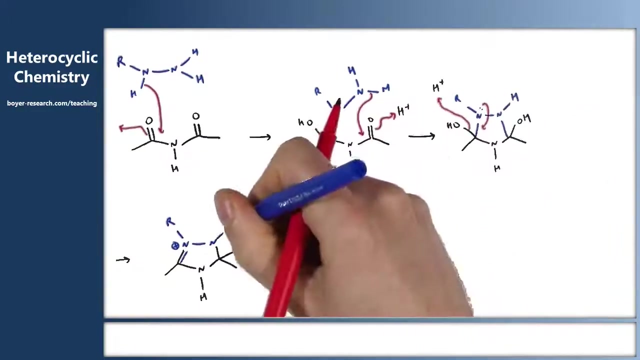 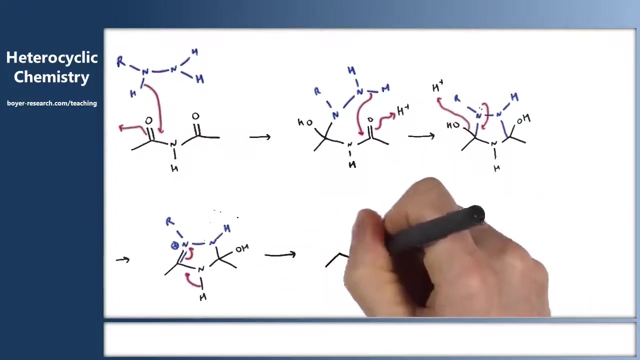 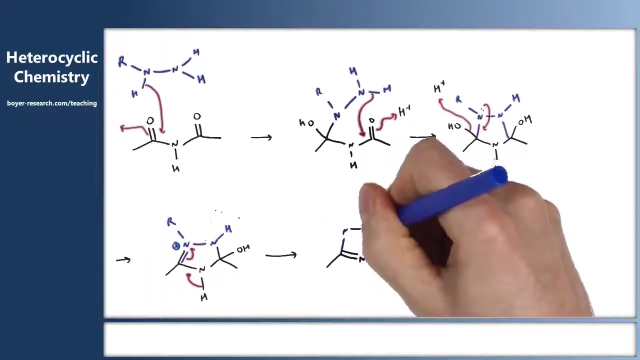 The lone pairs come in, They promote the loss of OH, Um Minus Promote by an H-plus. That gives us an iminium species which is neutralized by the loss of a proton, And we can repeat that process to give us the final aromatic heterocycle. 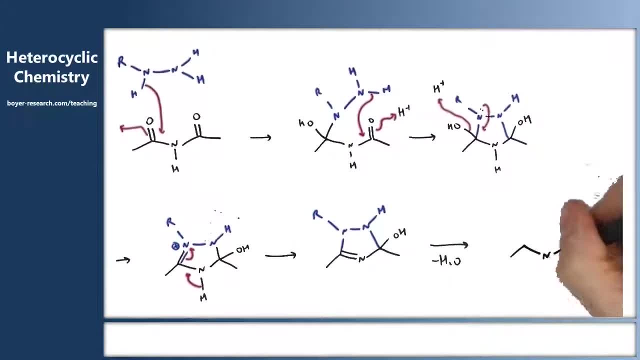 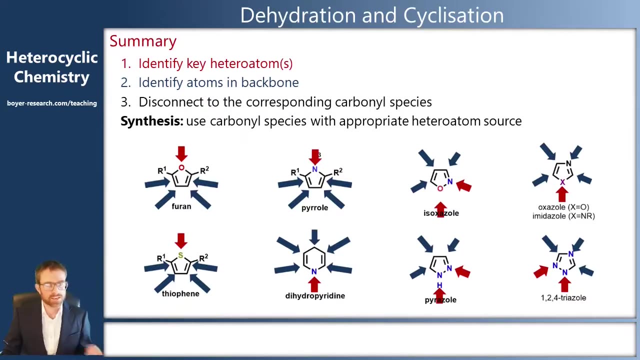 What we've seen is several different reactions, all of which have the same strategy. If we want to figure out how to make a heterocycle, we can identify the key heteroatoms that we know are going to need to provide, and then what that leaves in terms of the backbone.